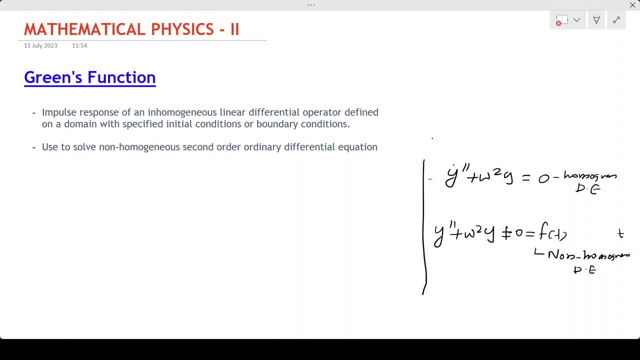 problem with a specified initial condition or a boundary condition. Okay, So normally this Green's function we just represented as in terms of g, it is g of x, t, where x and t are two different variables, which is, and the g Green's function is depend on these two variable, x and t, And this 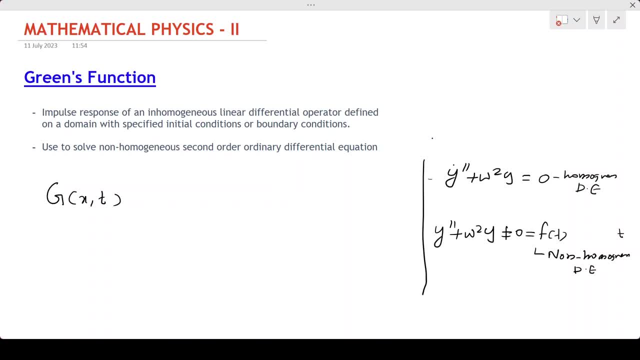 function is proposed by George Green in 1820s and he has described. this function is a method to solve a non-homogeneous second order differential equation. Okay, So here we see how do we execute this Green's function as a tool. And here let me just take an example of non-homogeneous 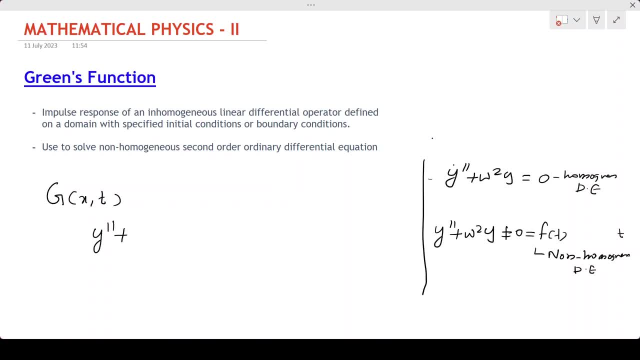 differential equation of this particular form: y double dash plus omega square y is equal to f of t. Okay, And keep it as equation number one. So this is my equation number one: y double dash, omega square y is equal to f of t. And this y double dash, as you know, this is d square, y by dx square. 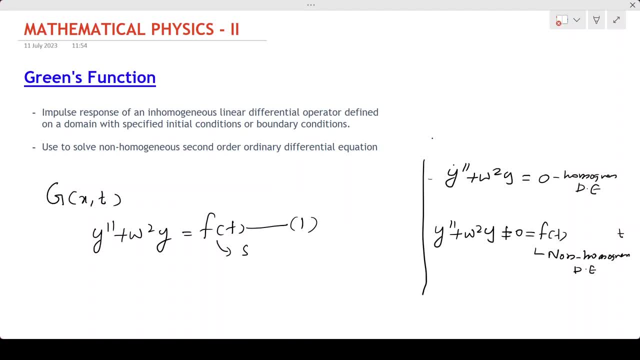 y. So that is an f of t. we call a source function. Okay, We call a source function or force function, And this function is actually triggering a particular particle, if you take a single particle here, So if you trigger a force on this particle and corresponding to with respect to that. 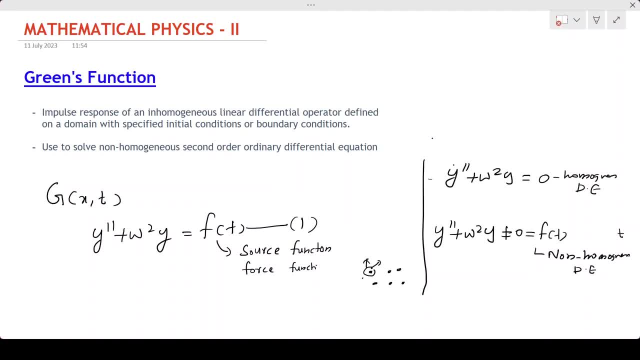 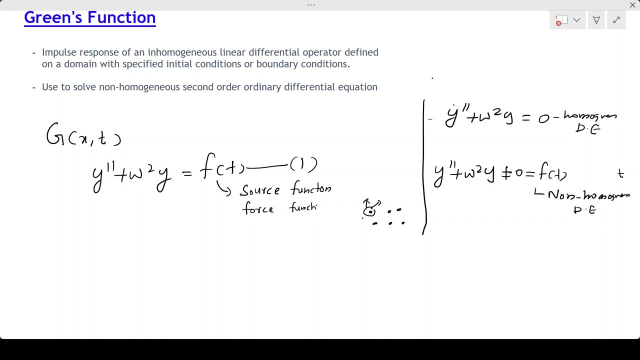 force, there will be a movement towards this particle and there is an impulse will be associated with that. So this force function we can also call as an impulse function in that case. Okay, So now, if you want to find the solution of this non-homogeneous second order differential equation, 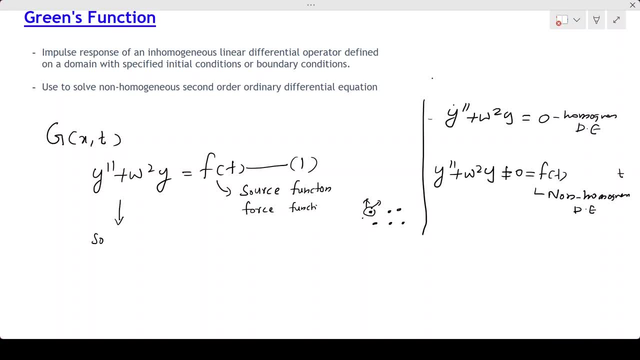 So we basically the solution of this equation means: So the solution of this equation means you need to find what you need to find- y of x, Okay. So the solution of the equation means you are actually trying to find that, Okay. 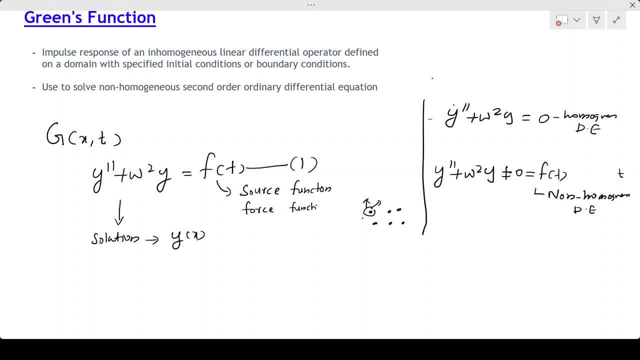 So what we are going to find: y of x, the find, the particular function that is depend of x or t. Okay, So that is the solution of a particular, this particular or differential equation. Now, if I just replace this equation y of x with respect to, or y of x, t, w ith respect. 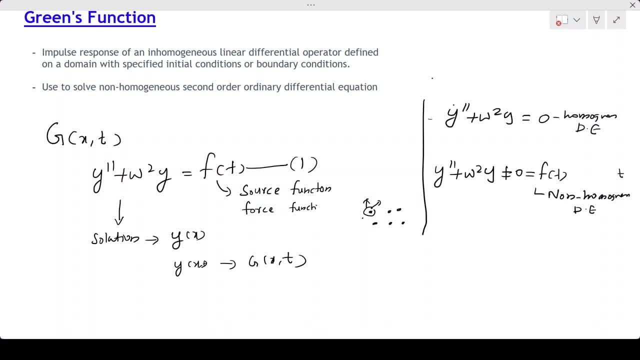 to g of x t, where g of x t is already said that it is a Green Function representation, Okay, And there is a specialty, or the property of that version of here is expression equation, okay, Okay. And so what we have to do is We are going to- we have a quicks, tenía lした. 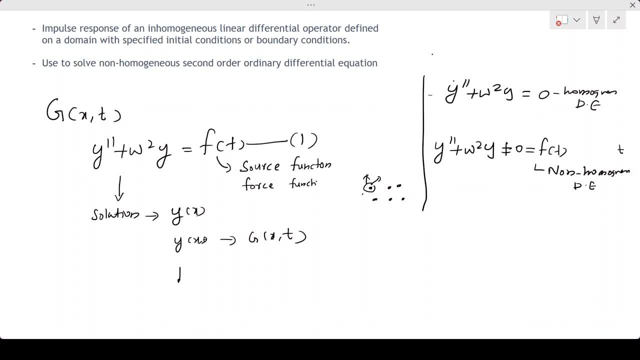 counter. So we are going to, we are going to actually explain the S and by and large, and then over Packer Green's function, that lg of xt is equal to delta x minus t. lg of xt is equal to delta x minus t where delta x minus t is a Dirac delta function. and you know the speciality of a Dirac delta. 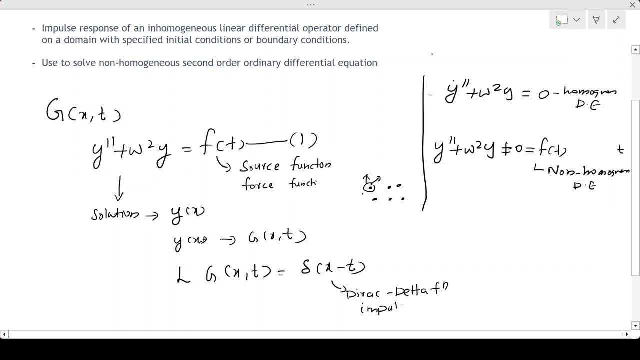 function, Dirac delta function, also called as impulse function. okay, which, having only one, only at a single point, is as the maximum value in all other point this Dirac delta function has a value will be zero. So all other point left, all other point, it has a zero value and we can see. 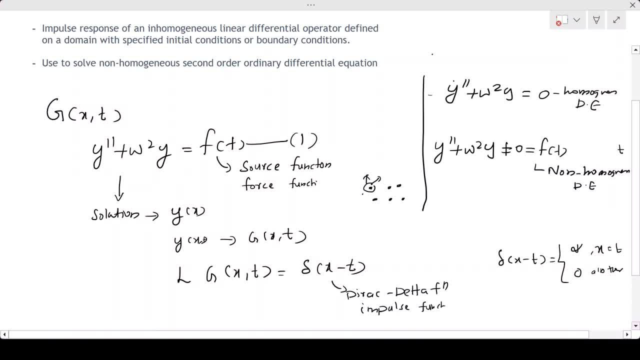 that this is an impulse function. Impulse function means on a sudden you can see that this is a Dirac delta function. So Dirac delta function, also called as impulse- All of a sudden you are actually applying a force and corresponding to that force. 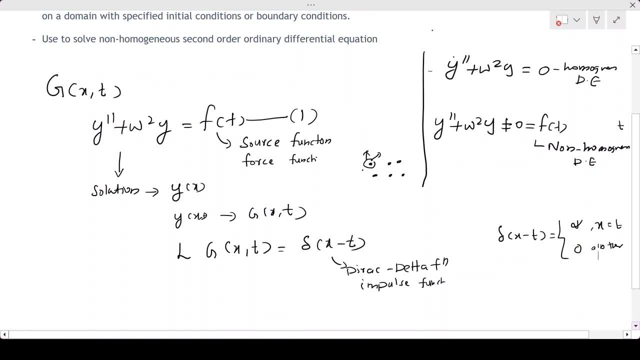 they are getting a sudden impulse or current response you are getting So, which we can actually represent as a Dirac delta function. The details of the Dirac delta function you have already covered in your mathematical physics 1 course, So I am not going very detailed into that. 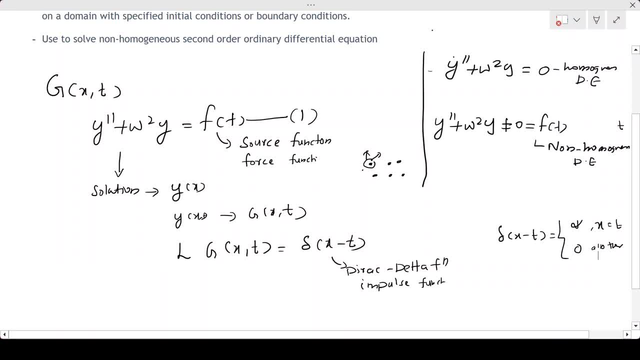 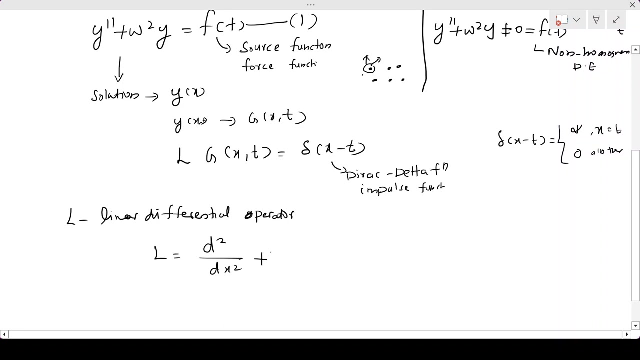 But what I am trying to say is that here you can see that L, where L is a linear differential operator, okay, So L is a linear differential operator. okay. For example, let me just take L as d square by dx square plus omega square, as a. 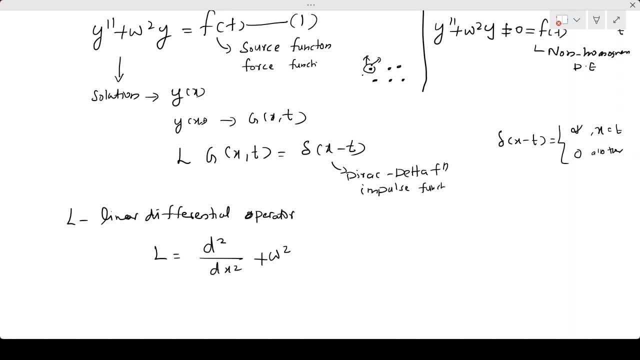 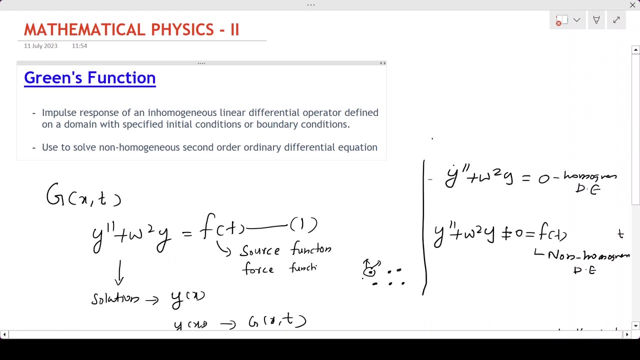 linear differential operator which is operating on a green function And the resultant will be a Dirac delta function. And that was the statement. also Here we have stated that Green's function is an impulse response of an inhomogeneous linear differential operator. 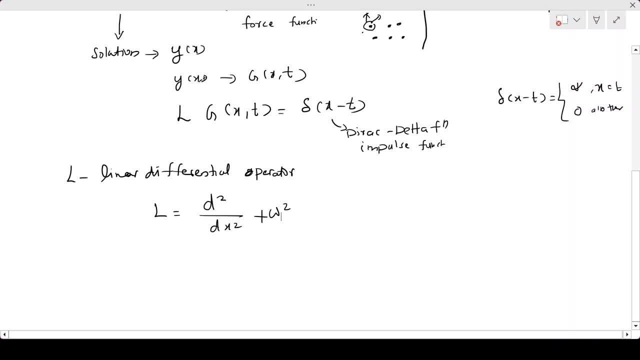 That inhomogeneous linear differential operator that is d square by dx square plus omega square, And that impulse response, we can treat it as an impulse function or the Dirac delta function. So if a differential operator operating on a Green's function 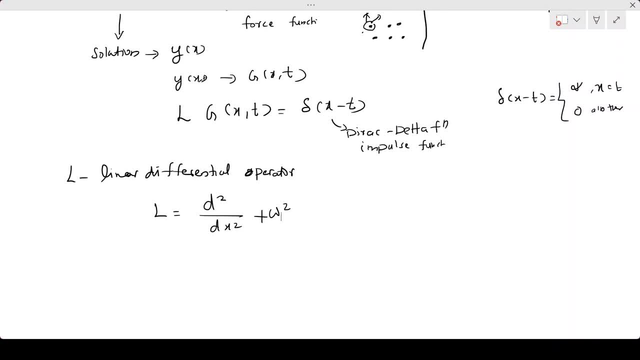 the corresponding result will be a Dirac delta function. That is one of the property Of a Green's function, And there are many other properties also there for Green's function that we will be discussing in the next lectures. okay, So this equation, also an important one, keep it as equation number two, okay. 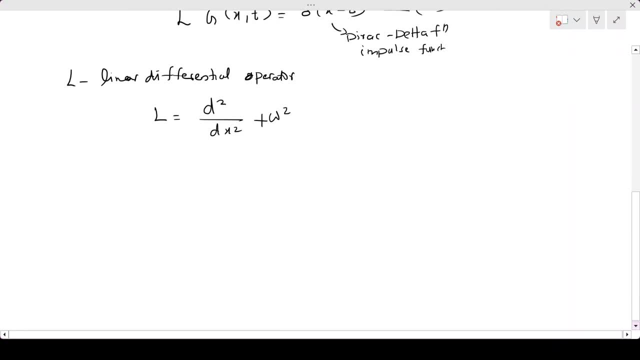 Now let me come back to our discussion. So we were discussing from equation one. from equation one, we know that there is an f of t plan. Equation one means y double dash plus omega. square y is equal to f of t. 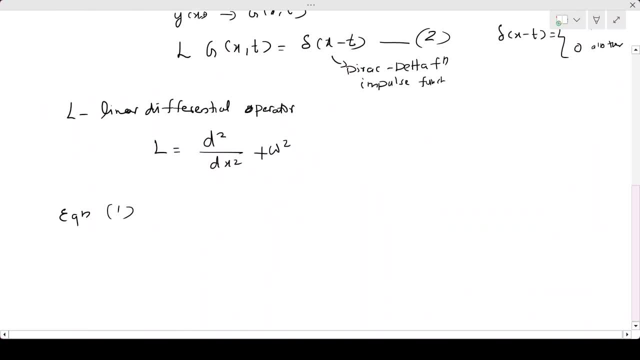 And where f of t, we specified that f of t is a. what f of t is? a force function or impulse function? So we can say that in equation one. in equation one, if I replace f of t with delta x minus t at, x is equal to t. okay, 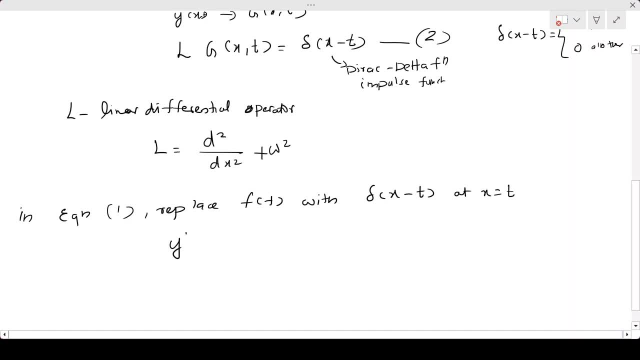 And then that is equal to f of t plus omega square y is equal to f of t. And then that is equal to f of t with delta x minus t at x is equal to t. okay, That equation becomes what That equation becomes: y double dash plus omega square y is equal to delta x minus t. you will be getting okay. 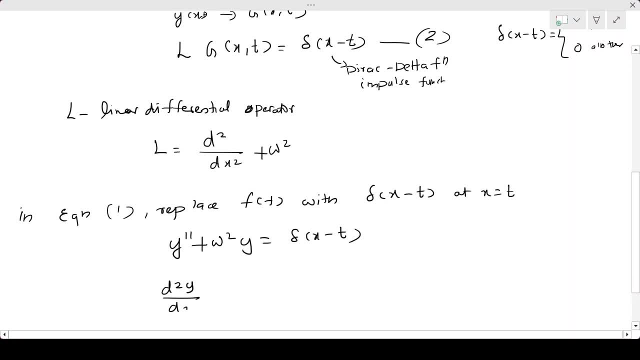 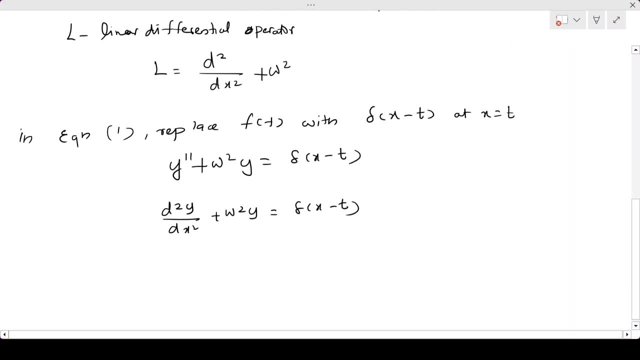 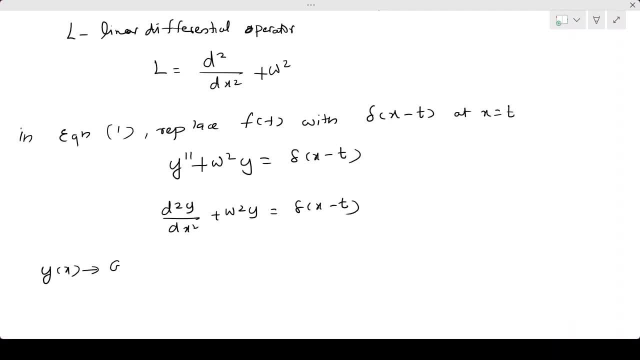 what It is, the solution of the differential equation which I just convert in terms of g of x t So that this equation becomes what This particular equation becomes: d square g of x t divided by d x square plus omega square g of x t, that is equal to delta x minus t. And if I take 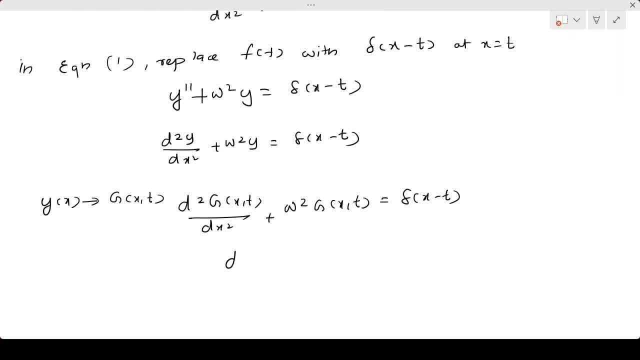 the operator out. So operator out means. so I am just taking d square by d x square plus omega square outside of this bracket and we have g of x t, delta of x minus t And now this operator. we already specified that. what is this operator? that is l, g of x t and that is equal to delta x minus. 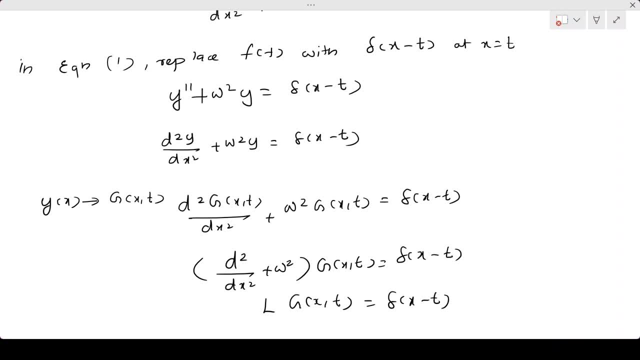 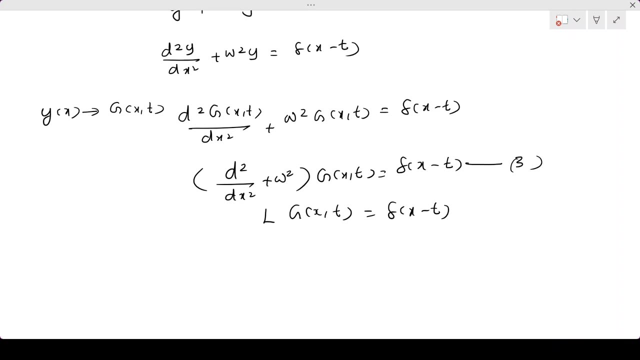 t. So here you can see that this operator l is already we specified. l is what d square by d, x square plus omega square. So l g of x t is equal to what Delta of x minus t. So I am just keeping this particular equation as equation number 3 for convenience. now 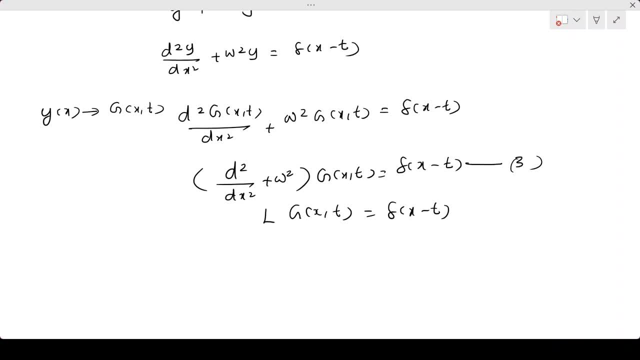 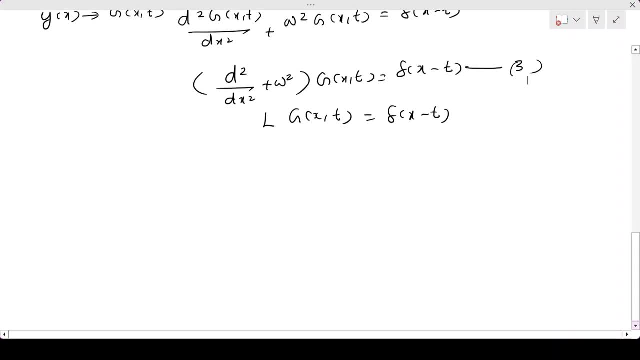 So this equation number 3 is d square by d, x square plus omega. square g of x t is equal to delta x minus t. So if I specify the solution of the non-homogeneous equation or solution of equation number 1 as in terms: 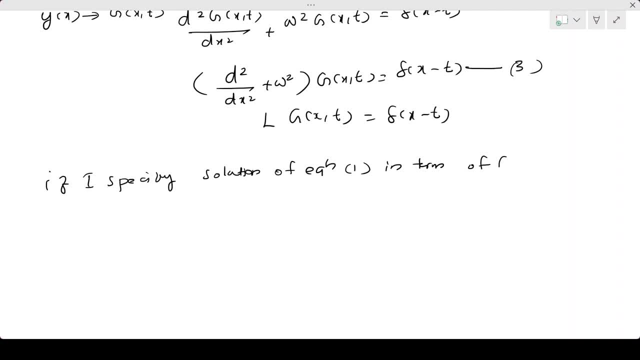 of or in terms of Green's function, so that I can represent. so that will be: y of x is equal to integral 0, to infinity, g of xt, f of t, dt. so this is equation number 4. so equation number 4 is the solution of the equation number 1, that is a non-homogeneous second. 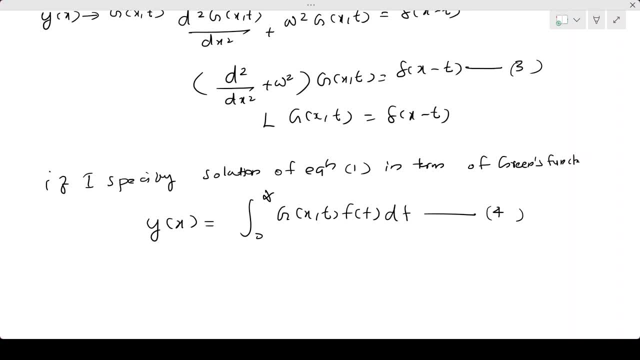 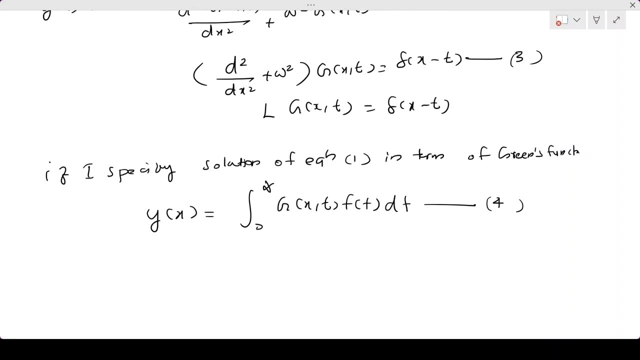 order differential equation. we have specified y, double dash plus omega square y is equal to f of t. so this is a possible solution in terms of Green's function. that you can see now. now what I am checking that, whether. so let me just check that. check whether the f 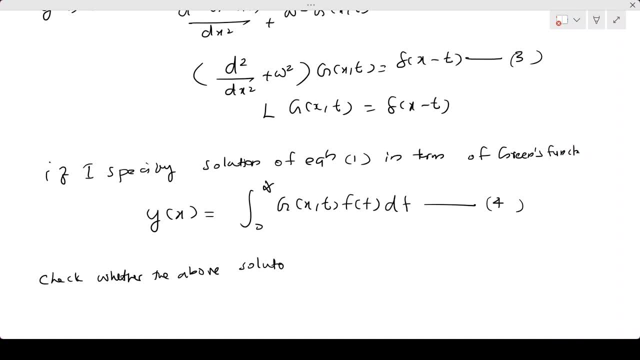 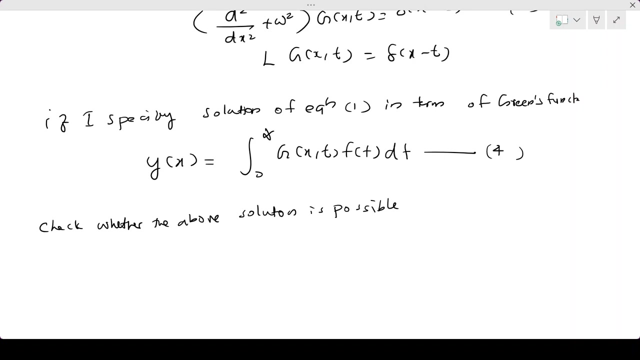 of t and both solution is a possible one or gives result, which means If I substitute y of x into that equation number 1, I will get the solution as f of t. for example, you can, if you take that first equation, equation number 1, omega square y. 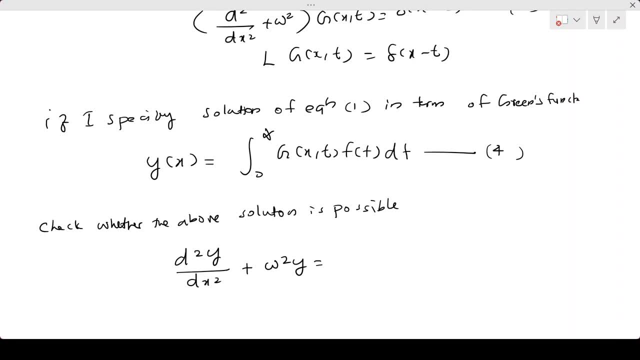 square y is equal to, so we all get that that is f of t, right? so if i substitute y of x is equal to this particular solution, 0 to infinity, g of x, t, f of t, dt, whether i am getting f of t or not. so if i am getting f of d as the solution, then i can directly say that this is the possible solution. 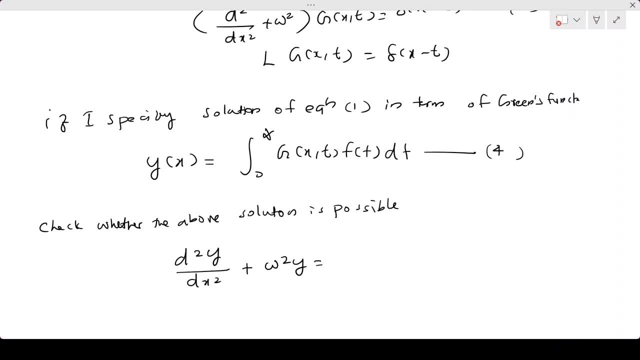 of that particular differential equation in terms of torture. so what i am doing is that i am just substituting. i am just substituting y of x as 0 to infinity g of x, t, f of t, dt, so that this equation becomes 1. let me just take the operator out side now. d square by d x square. 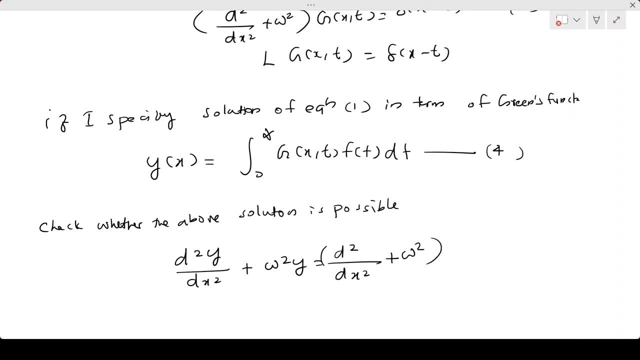 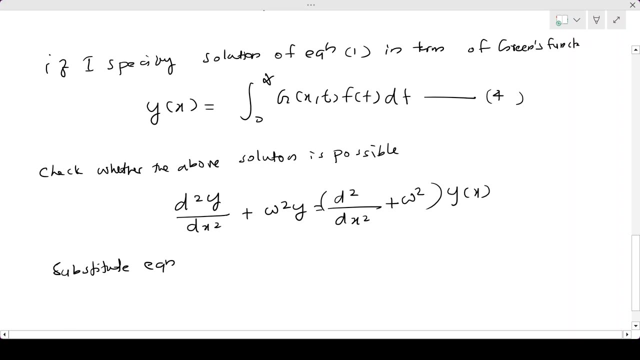 plus omega square. let me just take outside into y of x and 1: 1, 1 y of x. I can substitute as ok. so here I substitute equation number 4, so that this becomes what d square by dx square plus omega square into 0 to infinity: g of xt, f of t, dt. 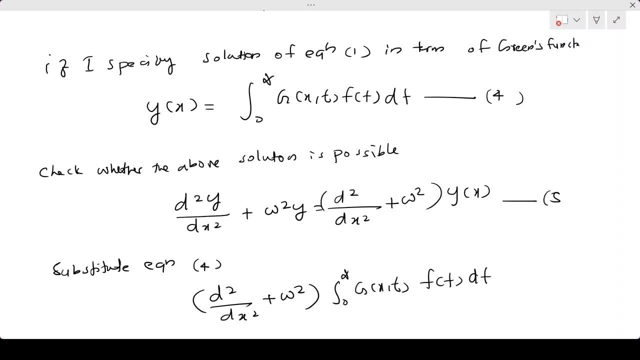 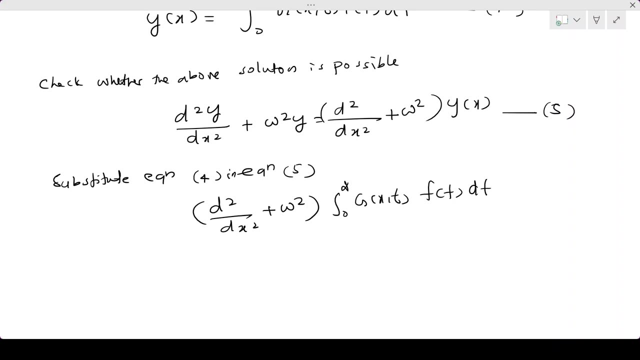 ok, so if I substitute, if I keep in equation number 5, in equation number 5, ok, so we will get correspondingly this solution. ok, and what will be the possible solution of this one, the possible solution of this one? 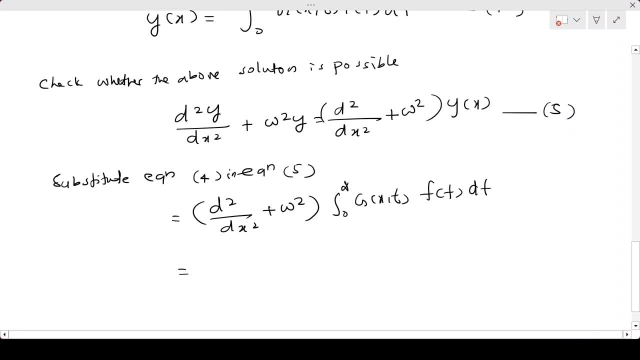 so you can get that d square by dx square. that is already. we know that that is l, l, so if I take that into instead, d square by dx square plus omega square g of xt, f, of t, dt, and we can see that from that. 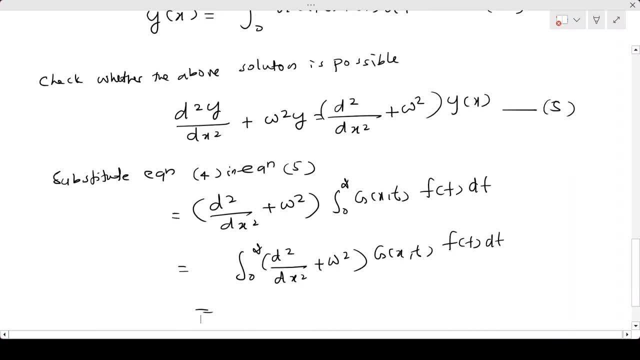 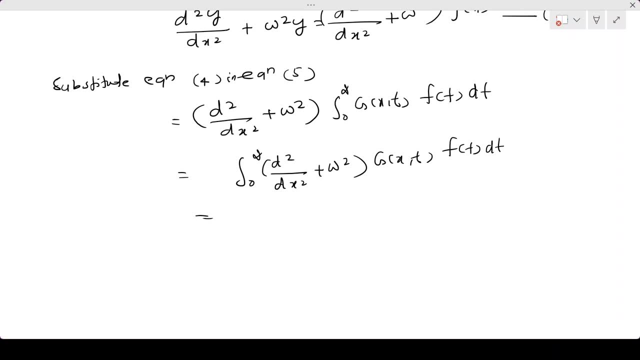 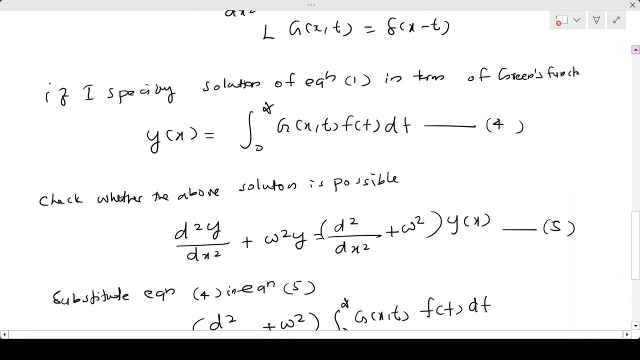 ok, ok, this is d square by dx square plus omega square into g of xt, f of t, dt. and we have seen that this particular portion has a solution in equation number 3, that is, equation number 3 says that d square by dx square plus omega square g of xt is what? 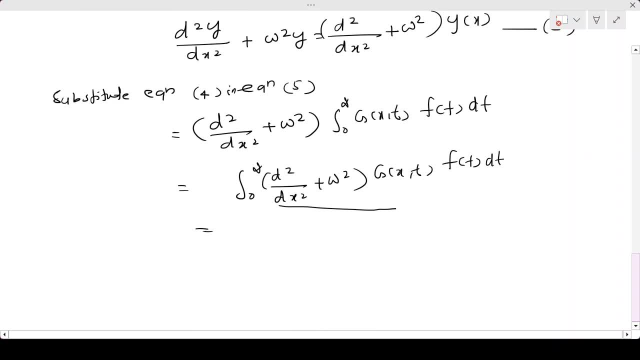 delta x minus t. so I can replace this part of the equation with what, this part of the equation with delta x minus t. so that is 0 to infinity. delta x minus t f of t, dt. ok, delta x minus t, f of t dt. 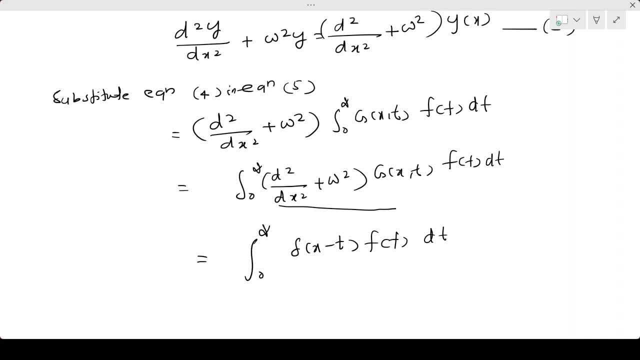 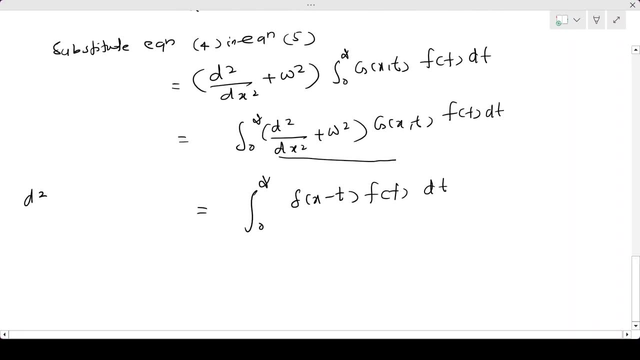 here at this point. so what is this one? so this is d square by ok here at this point. so this is d square by dx square plus omega square g of xt, f of t dt. so this is d square by dx square plus omega square g of xt, f of t dt. 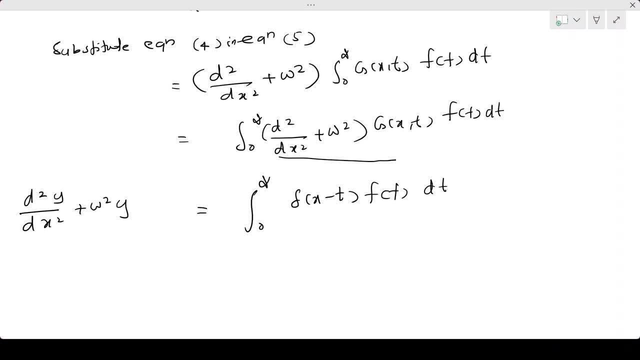 that is equal to delta x minus t, f of t. so we have, we have an identity relation that you would have studied in that you have studied in mathematical physics 1, so that identity relation says that if there is a function, if there is a function f of 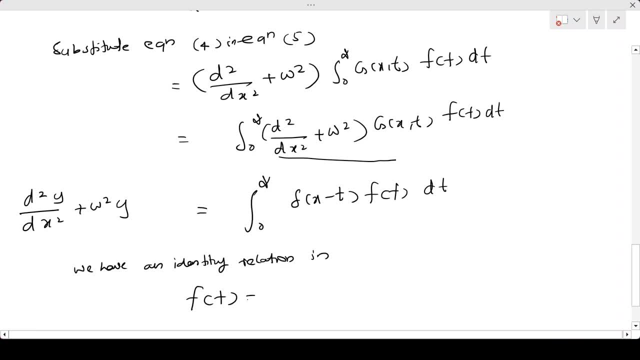 t that is equal to 0 to infinity delta. t minus t, dash, f of t, dash dt. ok, where delta is again Dirac delta function. so Dirac delta function has an identity relation that is: f of t is equal to 0 to infinity delta. t minus t dash, f of t dash is equal to dt. 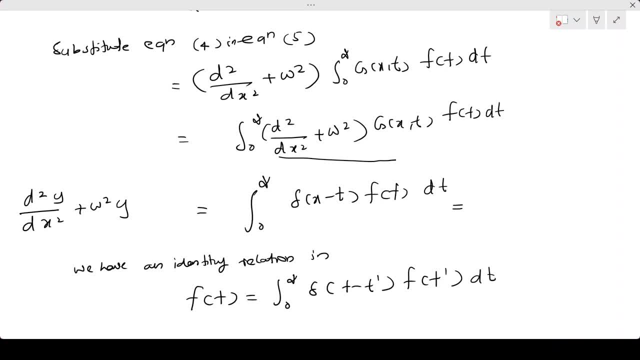 and that is what that will be the solution, what this will be: f of x. ok, by using this here, you can see that instead of t, dash, we have t, instead of t, we have x. so if you're considering this relation, 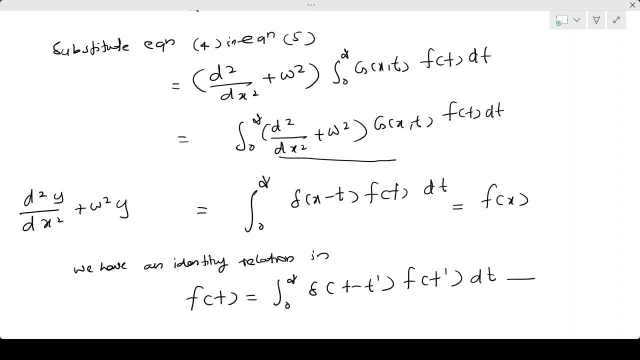 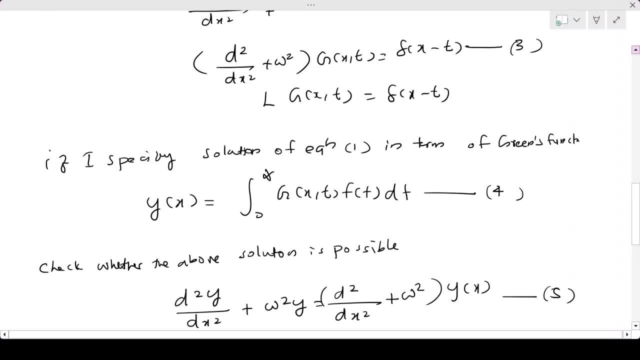 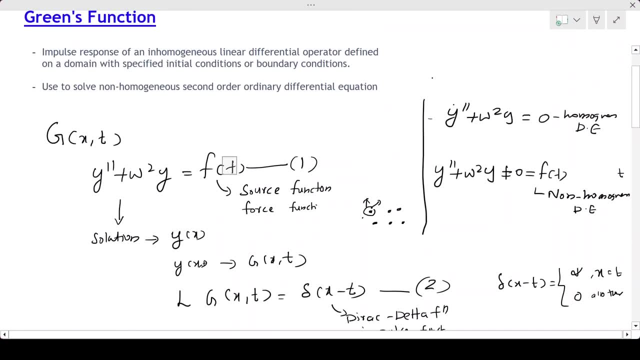 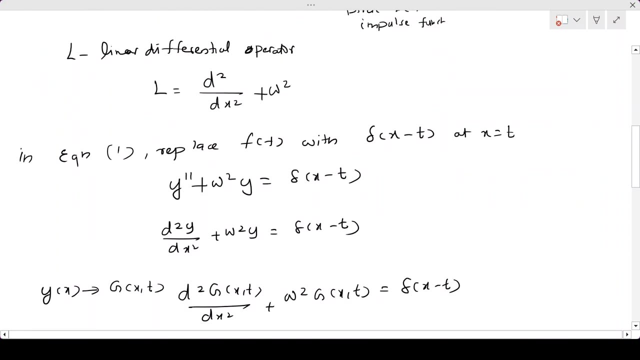 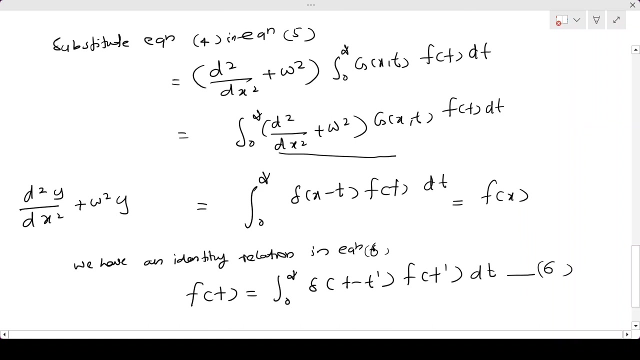 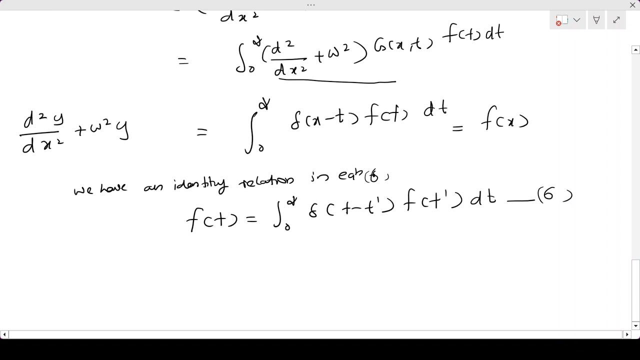 ok, f of x. ok, sorry, ok, there's a small correction here, so this will be possibly should be an x. ok, ok, so the solution will be what? so the solution will be what it will be: we will get as f of x. So what we have proven is that we have proven that if you. 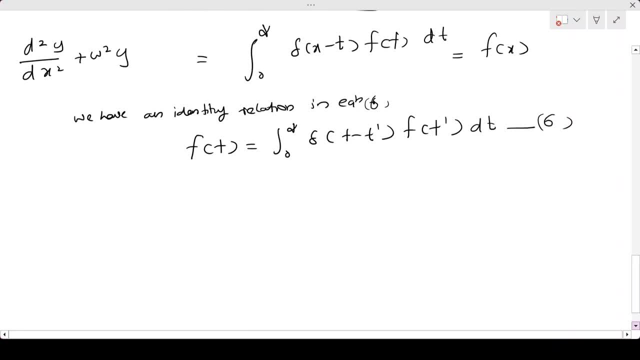 use the solution of y of x in terms of g of x, t. okay. So what we have proven is that d square y by dx square. So if you take the, if you have an equation d square y by x square, okay. So if you have an equation that is d square y by dx square as a differential, 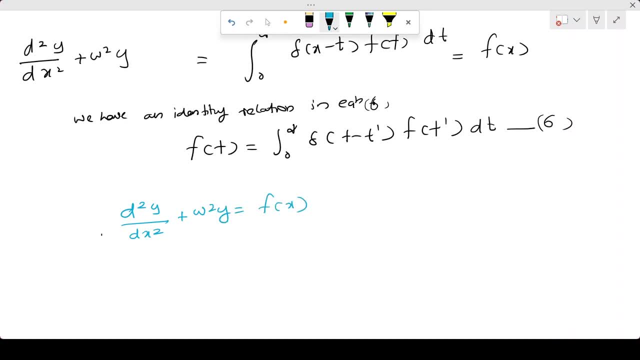 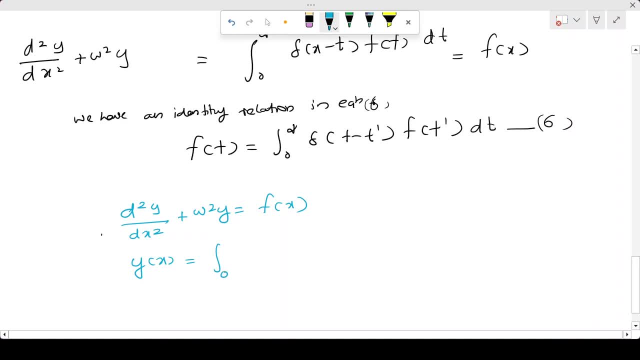 can be represented in terms of what? In terms of Green's function, g of x, t, f of t, dt. okay, g of x, t, f of t. So if you substitute y of x into this differential equation- and first one is a differential equation- the solution will be in terms of integral equation. 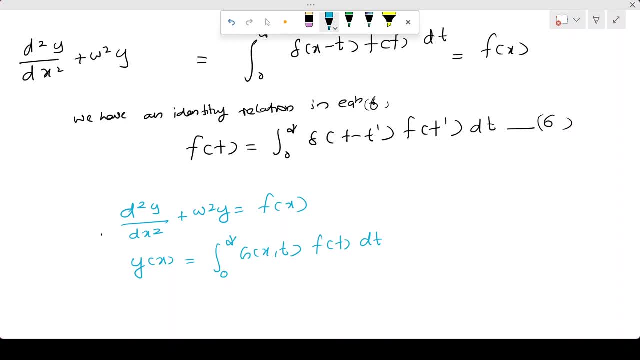 okay, And this integral equation. if you substitute into the differential equation, the characteristic of the solution will be f of x, t, f of t, dt. So if you substitute y of x into this equation, the corresponding solution will be f of x. that you will be obtaining. So that is what we. 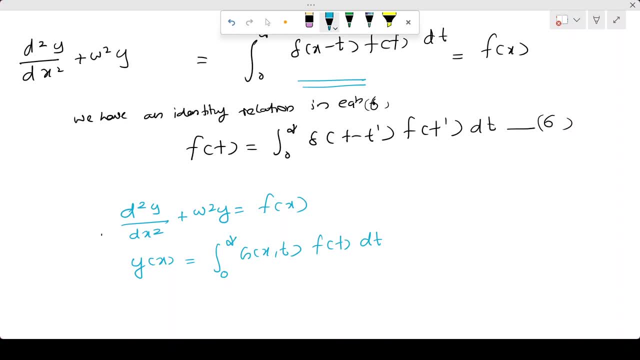 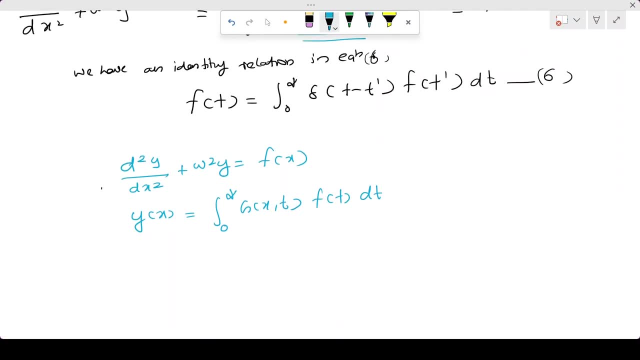 have obtained here. So we have get that. If you substitute the solution back to this equation, we are actually getting the solution of that particular. So we can actually we can actually represent this solution of this differential equation in terms of Green's function And we. 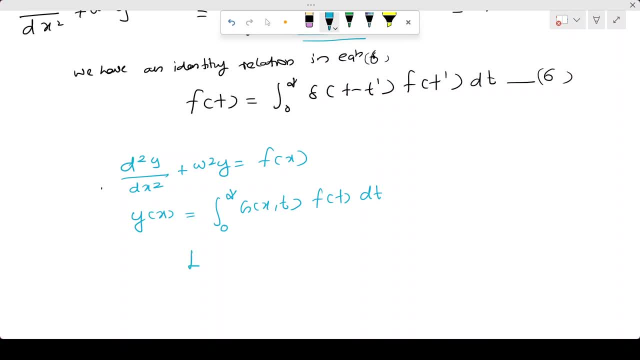 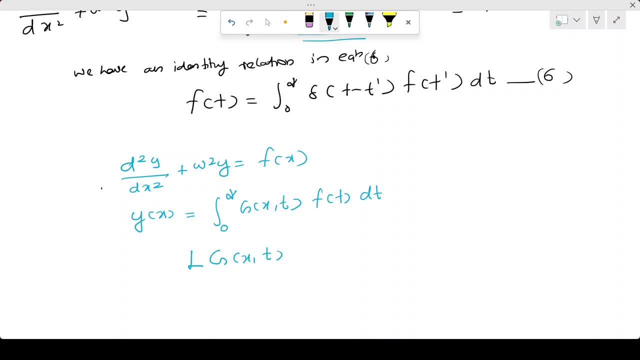 linear differential operator is operating on a Green's function, the corresponding solution will be- and that is, it is an impulse function that is a Dirac delta function. so this is one of the property of a Dirac delta function- Green's function as well. okay, and this is a solution. 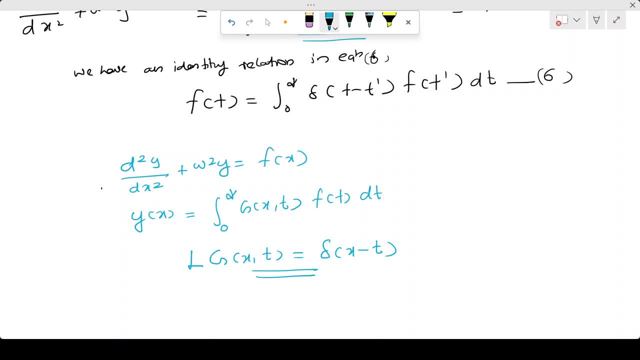 this is a possible solution. so if you know the Green function, if you know the Green function, if you substitute that into the integral equation, so you can actually get the corresponding solution of a non-homogeneous differential equation. so that is the point here. okay, so our main. 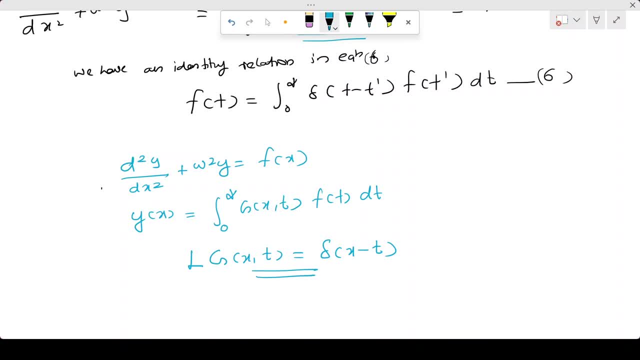 goal for this module is that to identify, or to identify the various method to identify the Green function. okay, to the way of finding Green function. so if you can find the Green function and you can substitute back into this equation, you can actually find the solution of a non-homogeneous. 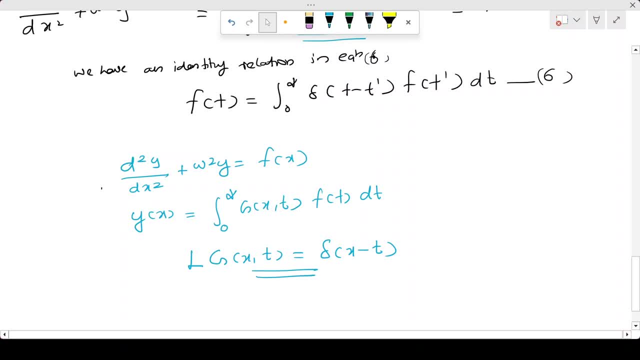 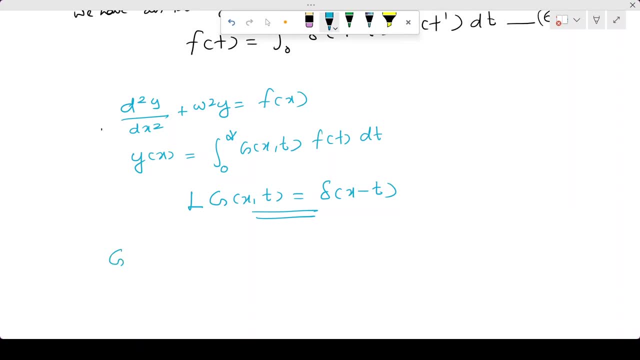 differential equation and also one point to end this session, that is Green function. Green function is a inverse response, as you can see that it is an inverse response of a system for a unit force applied, so we can say that it is an impulse response. that's what we can see now. this 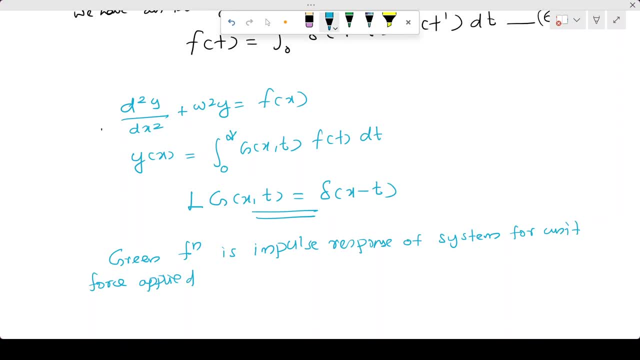 delta x minus t is a impulse function now. so when you are operating a linear differential operator on a Green function, correspondingly you are getting a impulse response. so we can see that it is an impulse response function or inverse response of a system for a unit force applied. 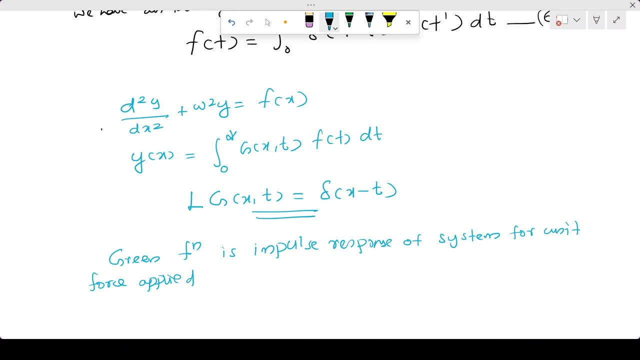 okay, so that's. that's it for today and the next session we'll be discussing regarding the one-dimensional Green's function and different properties of a Green function. how do we can say that a particular function to be Green function? so what are the properties to be satisfied? so that things we'll discuss in the next lecture. thank you.